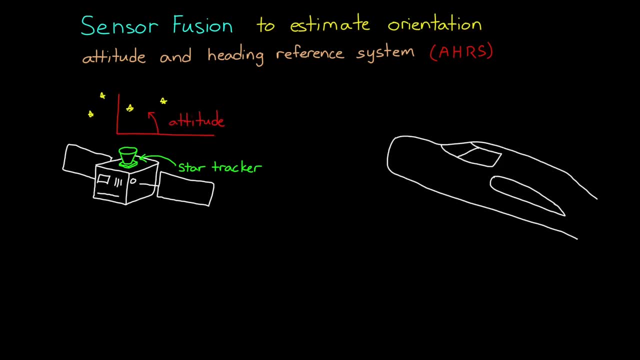 to estimate attitude relative to the inertial star field, Whereas an airplane could use an angle of attack sensor to measure orientation of the wing relative to the incoming free air stream. Now, in this video, we're going to focus on using a very popular set of sensors that you're going 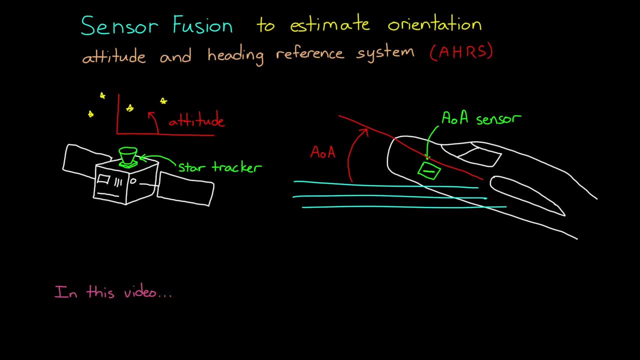 to find in every modern phone and a wide variety of autonomous systems- A magnetometer, an accelerometer and a gyro- And the goal of this video is not to develop a feature that will only work for a certain type of object. It's going to be to use a. 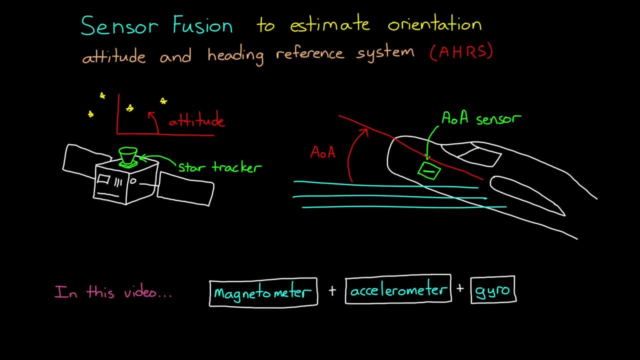 fully fleshed out inertial measurement system. There's just too much to cover to really do a thorough job. Instead, I want to conceptually build up the system and explain what each sensor is bringing to the table and a few things to watch out for. along the way, I'll also call out some 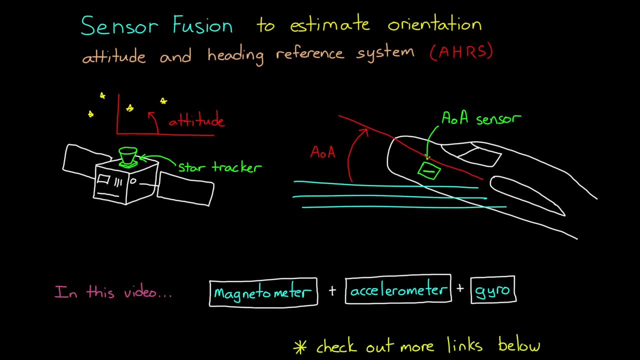 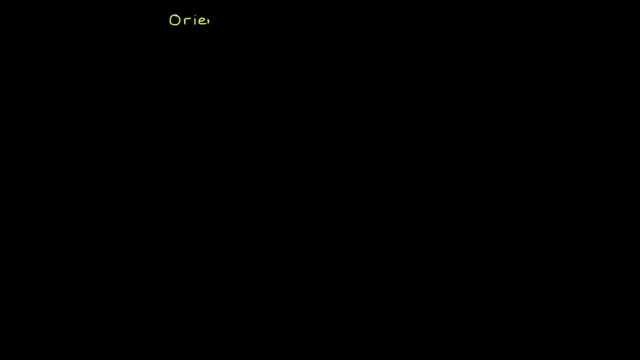 other really good resources that I've linked to below, where you can dive into more of the details. So let's get to it. I'm Brian and welcome to a MATLAB Tech Talk. When we're talking about orientation, we're really describing how far an object is rotating. 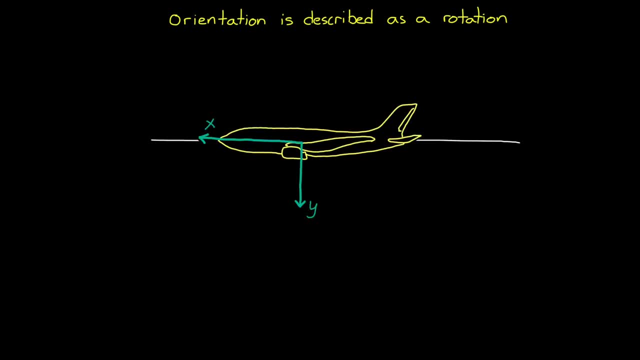 away from some known reference frame. For example, the pitch of an aircraft is how far the longitudinal axis is rotated off of the local horizon. So in order to define an orientation, we need to choose the reference frame that we want to describe the orientation against and then specify the rotation from that frame using some representation method. 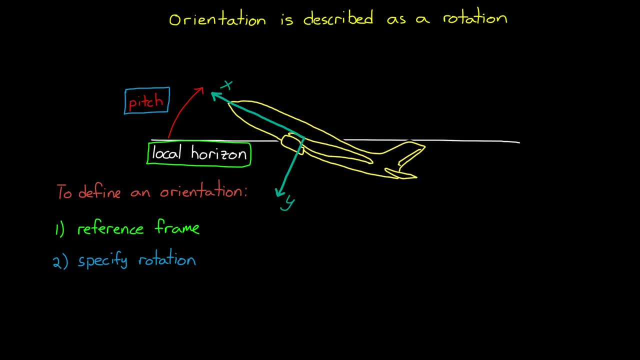 And we have several different ways to represent a rotation And perhaps the easiest to visualize and understand at first is the idea of roll, pitch and yaw, And this representation works great in some situations, For example, if we're talking about a plane, for example. 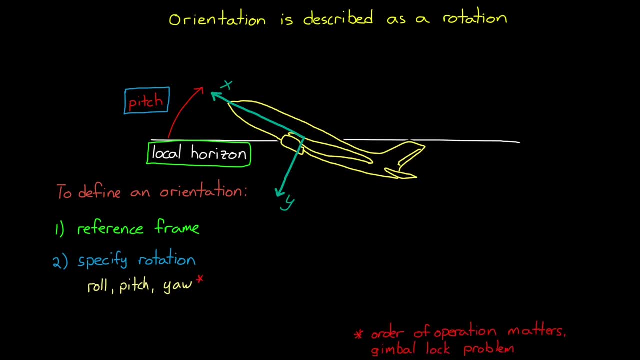 if we're talking about a plane, we're going to want to define a rotation in some situations. However, it has some widely known drawbacks in others. So we have other ways to define rotations for different situations, Things like direction, cosine matrices and the quaternion. Now the 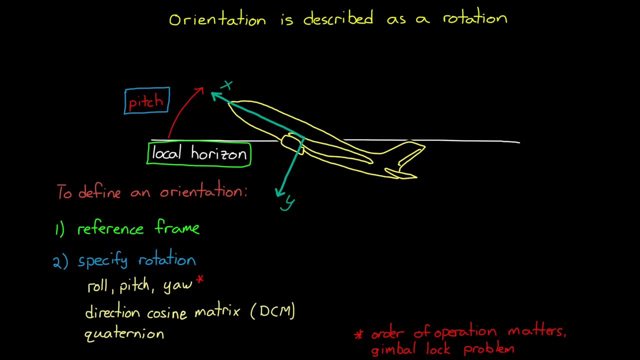 important thing for this discussion is not what a quaternion is or how a DCM is formulated, but rather just to understand that these groups of numbers all represent a three-dimensional rotation between two different coordinate frames: The object's own coordinate frame that is fixed to the 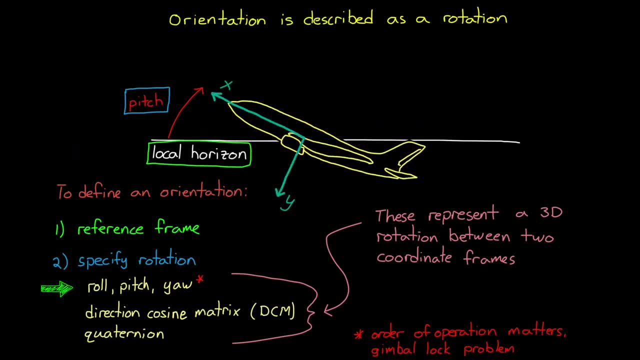 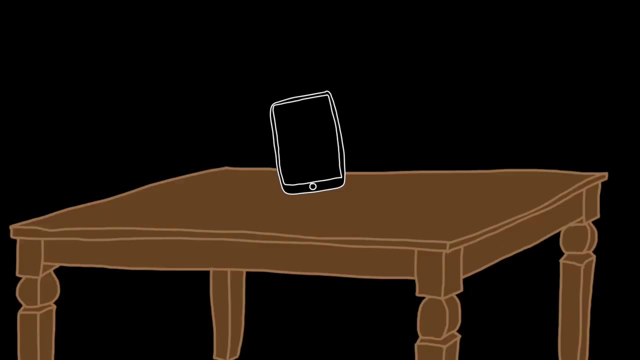 center of the plane. And it's this rotation, or these sets of numbers that we're trying to estimate by measuring some quantity with sensors. So let's get to our specific problem. Let's say we want to know the orientation of a phone that's sitting on a table, So the phone's body coordinate. 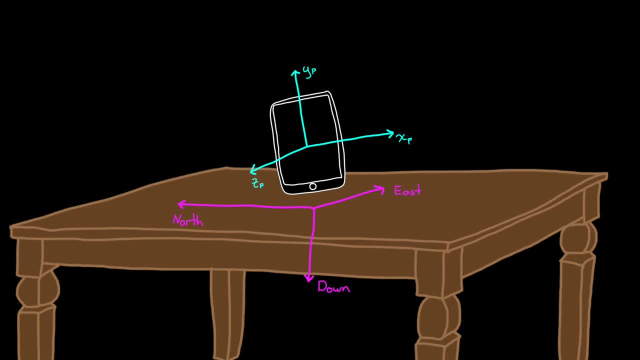 frame relative to the local north, east and down coordinate frame, We can find the absolute orientation using just a magnetometer and an accelerometer. Now, a little later on, we're going to use a gyro to improve accuracy and correct for problems that occur when the system is moving. 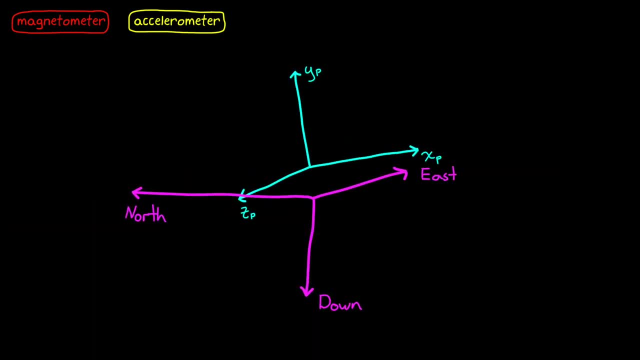 but for now we'll just stick with these two sensors. Simply speaking, we could measure the phone's acceleration, which would just be due to gravity, since it's sitting stationary on the table, and we would know that that direction is up, The direction opposite, the direction of gravity. 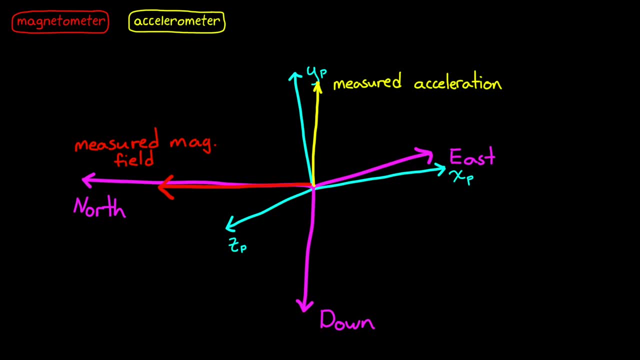 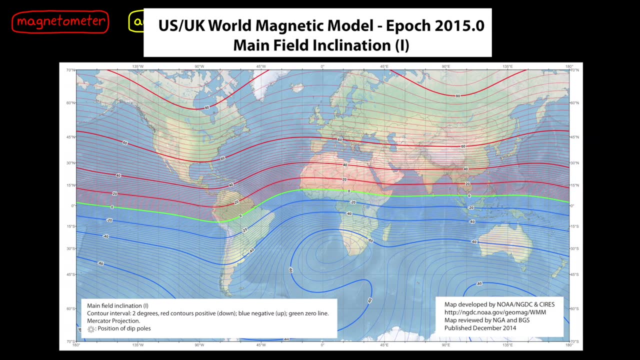 And then we can measure the magnetic field in the body frame to determine north. But here's something to think about: The mag field points north also points up or down depending on the hemisphere you're in, And it's not just a little bit In North. 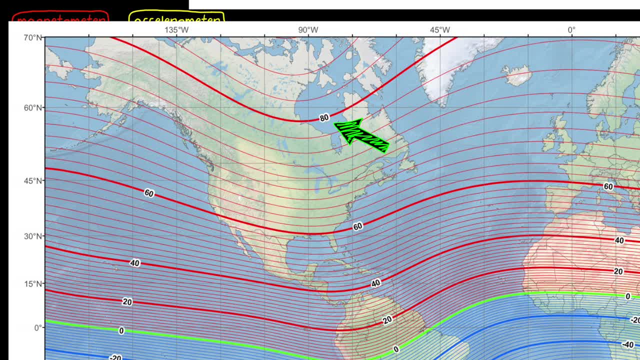 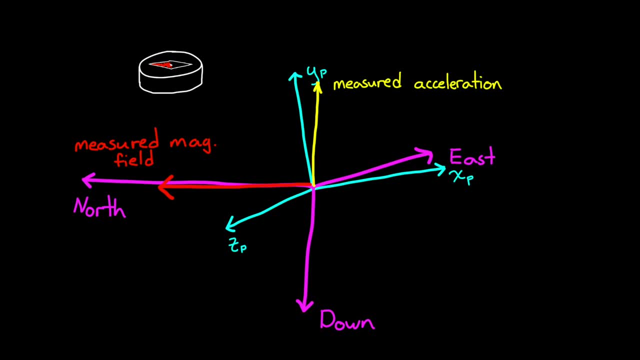 America, the field lines are angled around 60 to 80 degrees down, which means it's mostly in the gravity direction. Now, the reason a compass points north and not down is that the needle is constrained to rotate within a 2D plane. However, our mag sensor has no such constraint, so it's 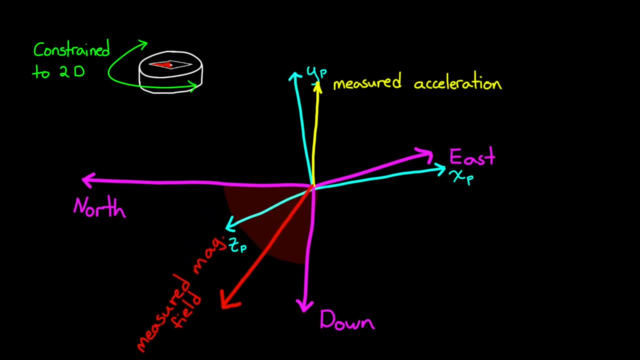 going to return a vector that's also in the direction of gravity. So to get north we need to measure the direction of gravity. We can start with our measured mag and excel vectors in the body frame. Down is the opposite direction of the acceleration vector and then east is the 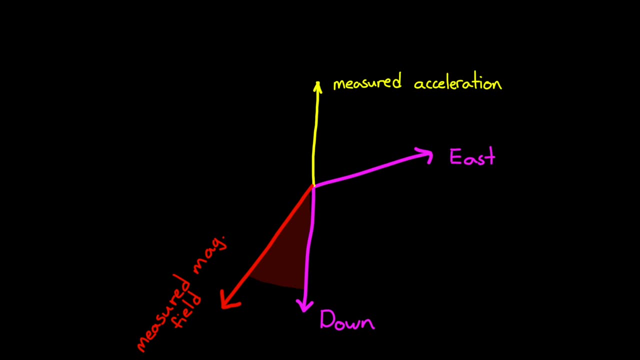 cross product of down and the magnetic field. And finally, north is the cross product of east and down. So the orientation of the body is simply the rotation between the body frame and the north east down frame And I can build the direction cosine matrix directly from the north east and 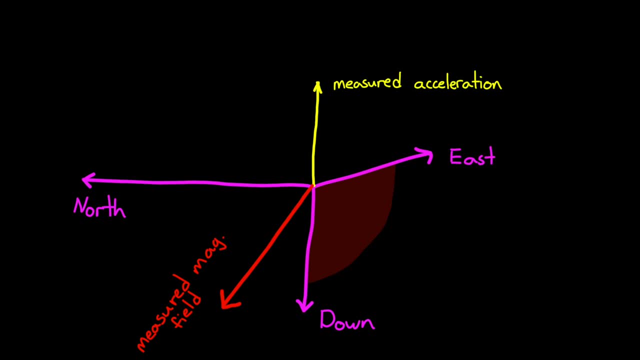 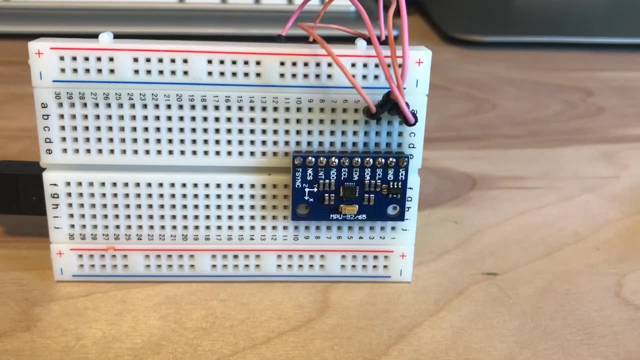 down vectors that I just showed you, So we can start with our measured mag and excel vectors in the body frame. Let's go check out an implementation of this fusion algorithm. I have a physical IMU- it's the MPU9250, and it has an accelerometer, magnetometer and gyro, Although for now we're 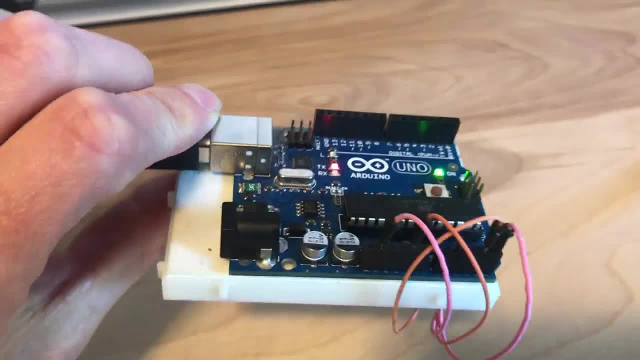 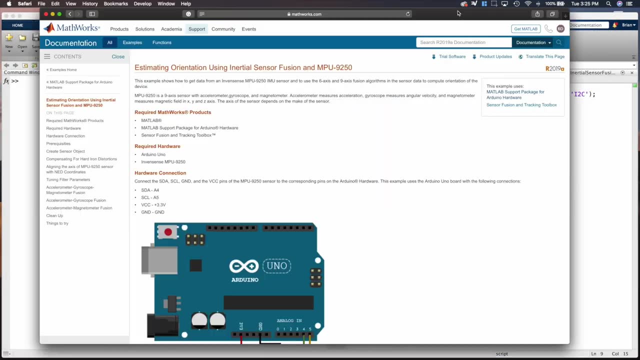 not going to use the gyro. I've connected it to an arduino through I2C, which is then connected to MATLAB through USB. I've pretty much just followed along with this example from the Mathworks website, which provides some of the functions that I'm using and I've linked to below, if you want to do the same. 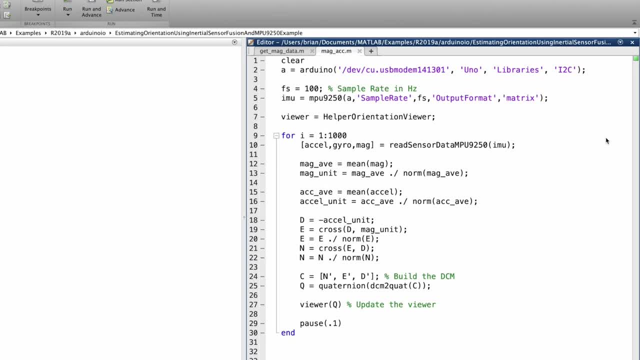 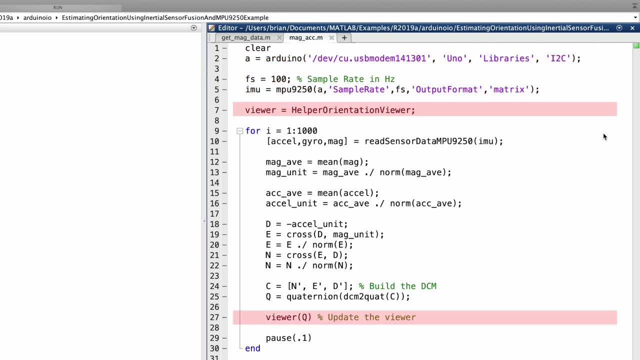 But let me show you my simple script. First, I connect to the arduino and the IMU and I'm using a MATLAB viewer to visualize the orientation, and I update the viewer each time I read the sensors. This is a built-in function with the sensor fusion and tracking toolbox. 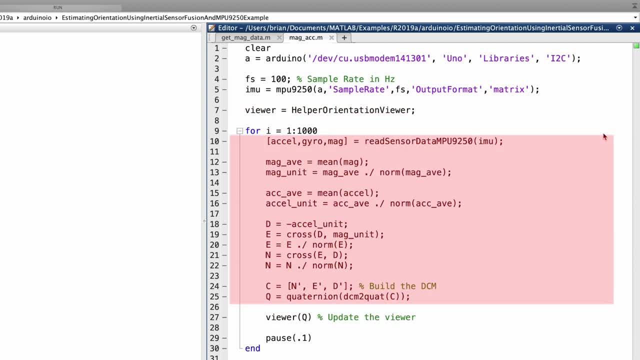 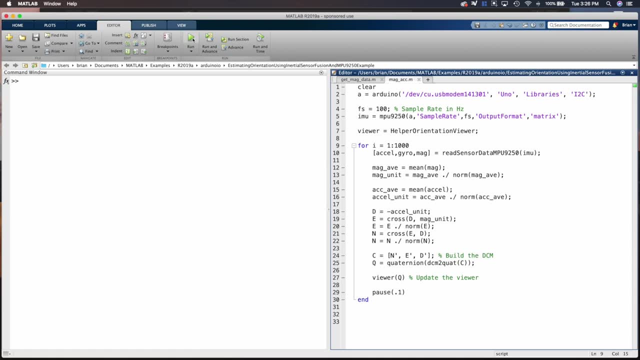 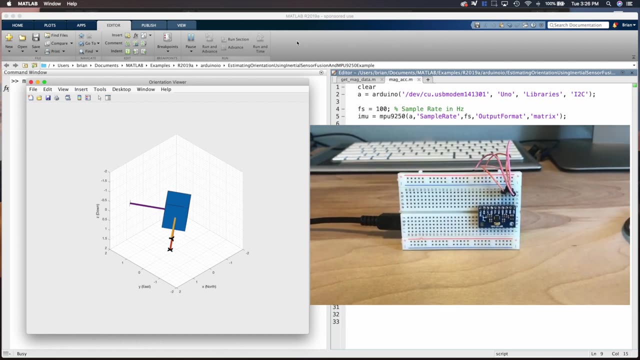 The small amount of math here is basically reading the sensors, performing the cross products and building the DCM, And that's pretty much the whole of it. So if I run this, we can watch the algorithm in action. Notice that when it's sitting on the table it does a pretty good job of finding down. 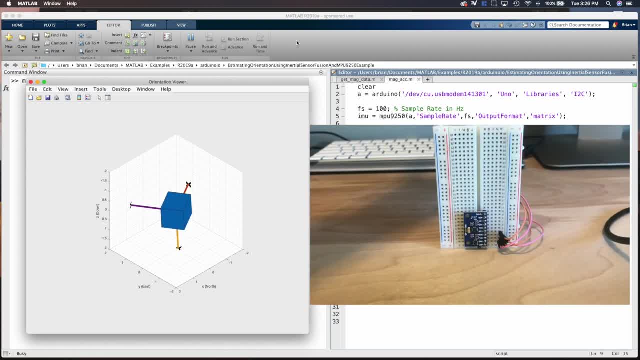 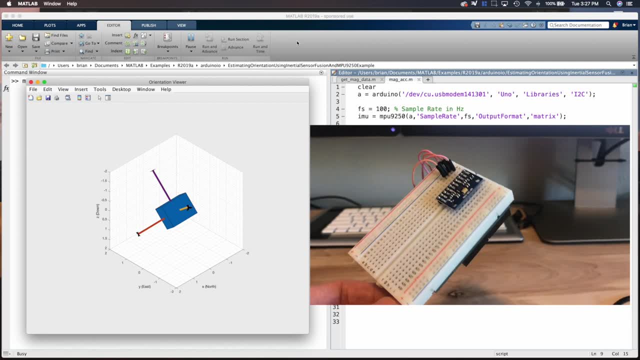 It's in the positive x-axis And if I rotate it to another orientation you can see that it follows pretty well with my physical movements. So, overall, pretty easy and straightforward, right. Well, there are a few problems with this simple implementation. I want to highlight 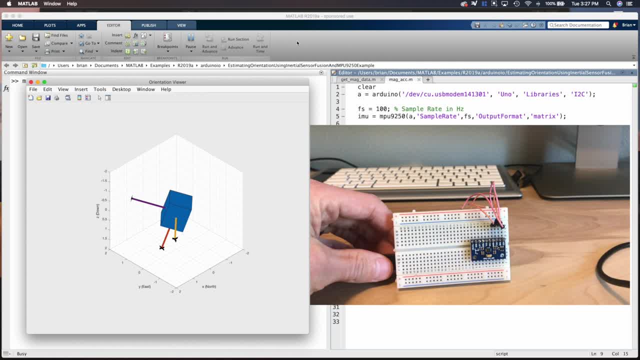 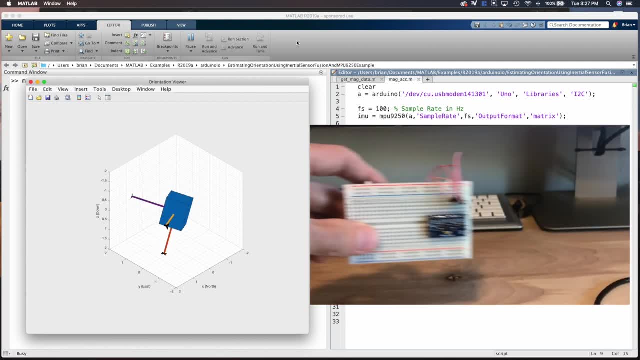 two of them. The first is that accelerometers aren't just measuring gravity, They measure all linear accelerations. So if the system is moving around a lot, it's going to throw off the estimate of where down is. You can see here that I'm not really rotating. 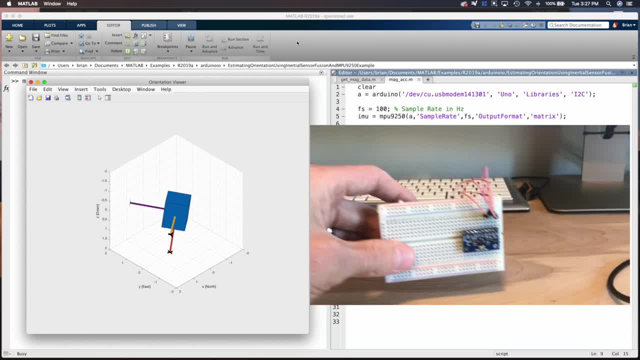 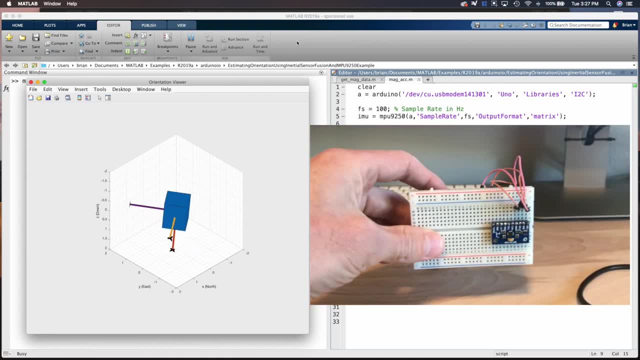 the sensor much, but the viewer is jumping all over the place, And this might not be much of a problem if your system is largely not accelerating like a plane while it's cruising at altitude, or a phone that's sitting on a table. But linear accelerations aren't the only problem. 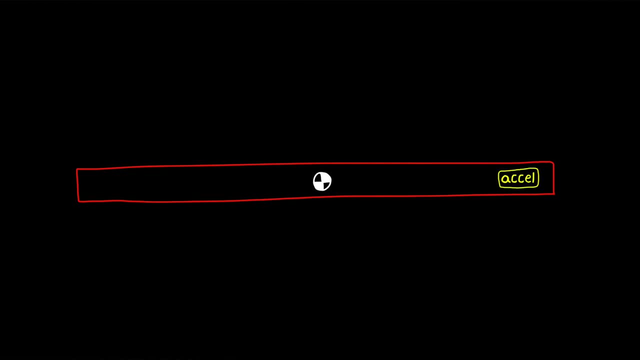 Even rotations can throw off the estimate, because an accelerometer that's not located at the center of rotation will sense an acceleration when the system rotates. So we have to figure out a way to deal with these corruptions. A second problem is that magnetometers are affected. 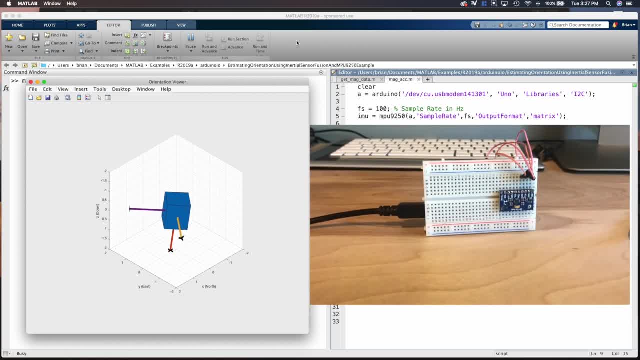 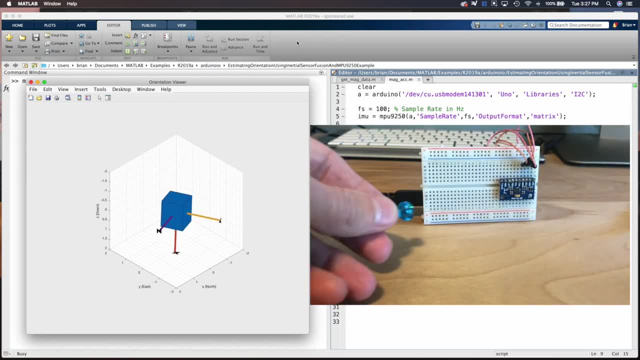 by disturbances in the magnetic field. Obviously, you can see that if I get a magnet near the IMU, the estimate is corrupted. So what can we do about these two problems? Well, let's start with this magnetometer problem. If the magnetic disturbance is part of the system and rotates with the 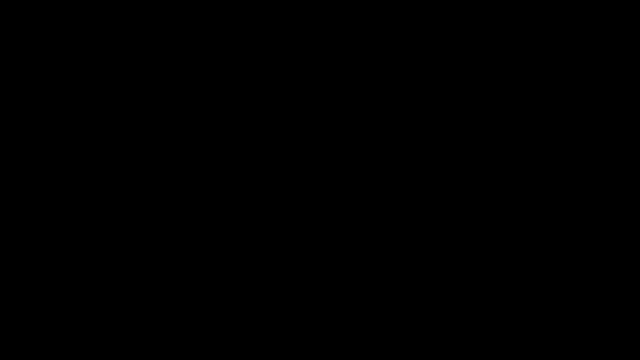 magnetometer, then it can be calibrated out. These are the so-called hard iron and soft iron sources. A hard iron source is something that generates its own magnetic field. This would be an actual magnet, like the ones in an electric motor, or it could be a coil that has a current running through it from. 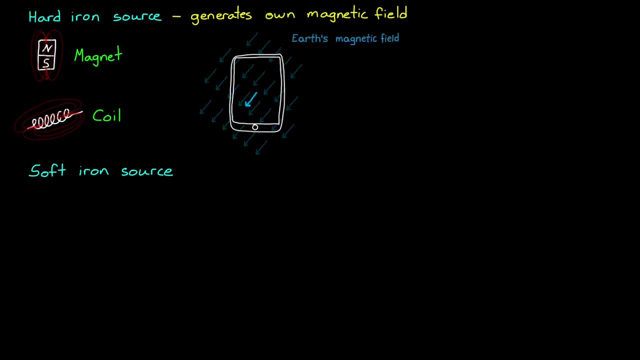 the electronics themselves. And if you tried to measure an external magnetic field, a hard iron source near the magnetometer would contribute to the measurement, And if we rotate the system around a single axis and measure the magnetic field, the result would be a circle that is offset. 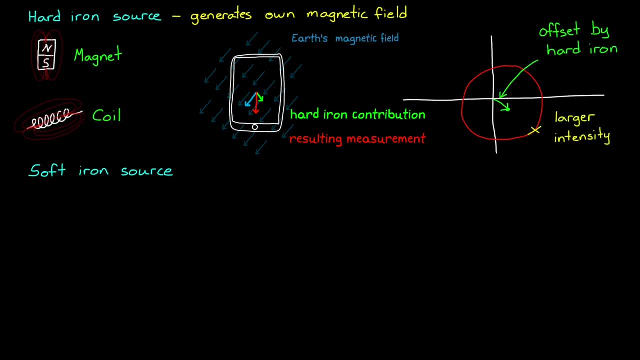 from the origin. So your magnetometer would read a large scale, but the result would be a circle: larger intensity in one direction and a smaller intensity in the opposite direction. A soft iron source is something that doesn't generate its own magnetic field, but is what? 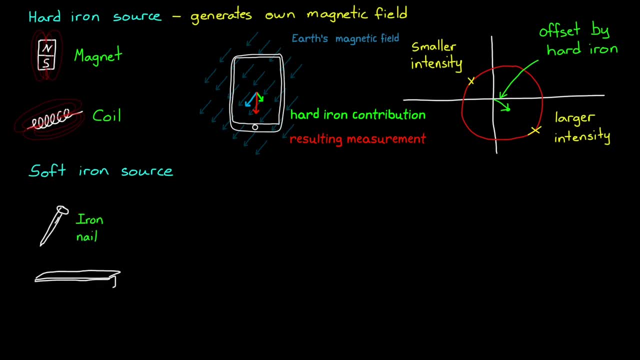 you would call magnetic. You know, like a nail that is attracted to a magnet or the metallic structure of your system. This type of metal will bend the magnetic field as it passes through and around it, and the amount of bending changes as that metal rotates. So a soft iron source that 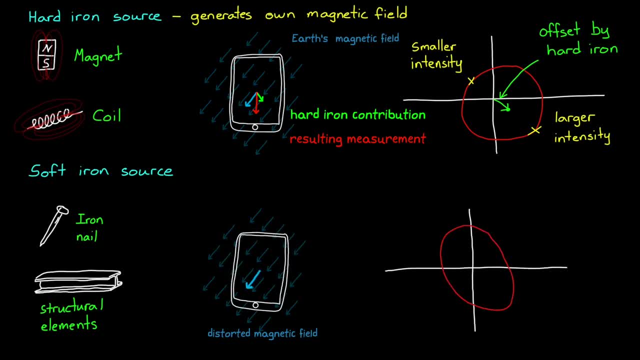 rotates with the magnetometer would distort the measurement, creating an oval rather than a circle. So even if you had a perfect, noiseless magnetometer, it's going to still return an incorrect measurement, simply because of the hard and soft iron sources that are near it. 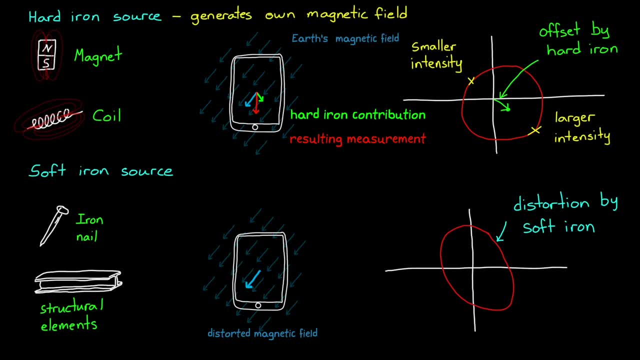 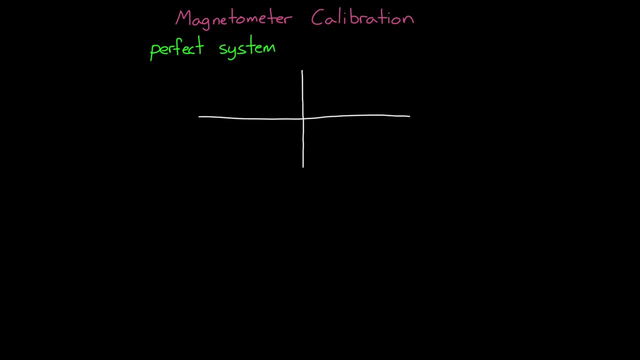 And your phone, and pretty much all systems have both of those. So let's talk about what we can do with calibration. If the system had no hard or soft iron sources and you rotated the magnetometer all around in four pi steradian, 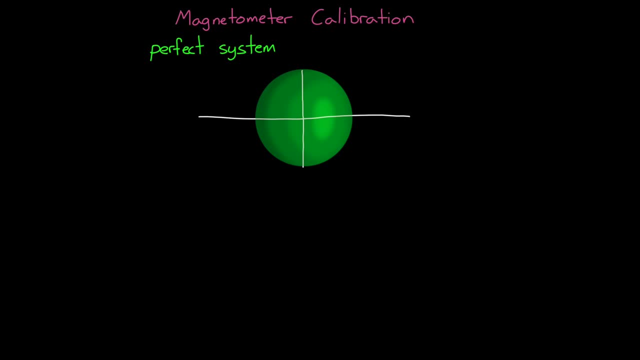 directions, then the magnetic field vector would trace out a perfect sphere with the radius being the magnitude of the field. Now a hard iron source would offset the sphere and a soft iron source would distort it into some odd shaped spheroid, If we can measure this distortion ahead. 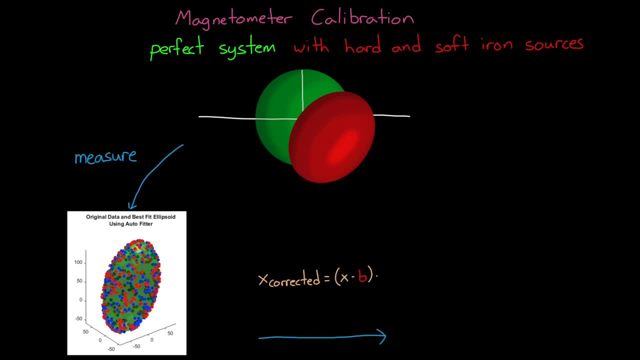 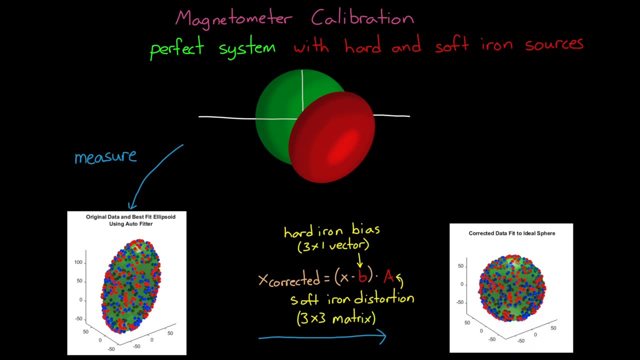 of time, we could calibrate the magnetometer by finding the offset and transformation matrix that would convert it back into a perfect sphere centered at the origin. This transformation matrix and bias would then change the direction of the magnetometer and the magnetometer would. 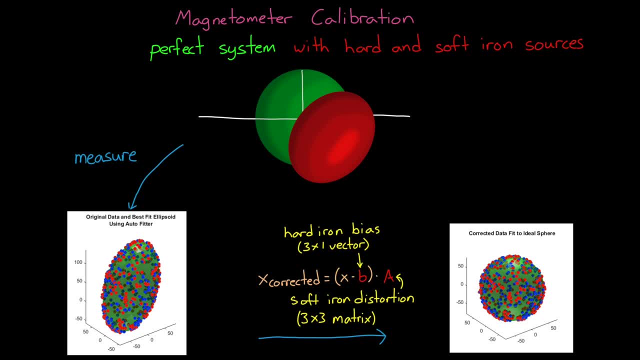 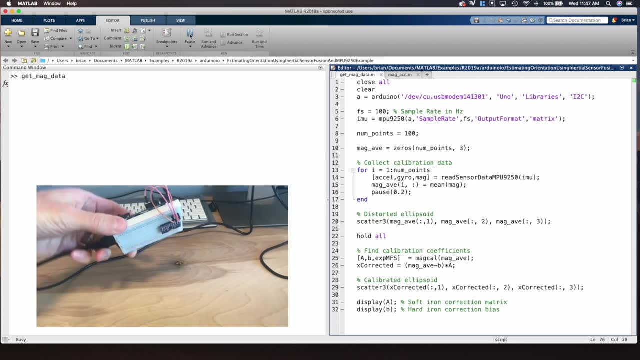 then be applied to each measurement, essentially removing the hard and soft iron sources. This is exactly what your phone does when it asks you to spin it around in all directions before using the compass. Here I'm demonstrating this by calibrating my IMU using the MATLAB function MagCal. 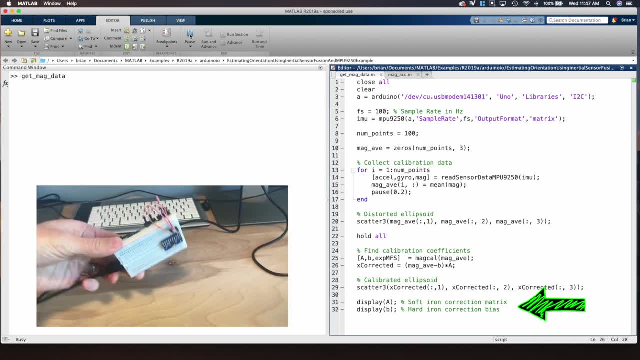 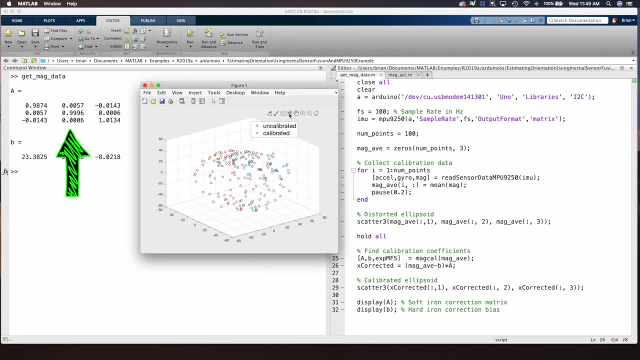 I'm collecting a bunch of measurements in different orientations and then finding the calibration coefficients that will fit them to an ideal sphere. And now that I have an A matrix that will correct for soft iron sources and a B matrix that route the hard undressed bias, I can add a calibration step to the fusion algorithm. 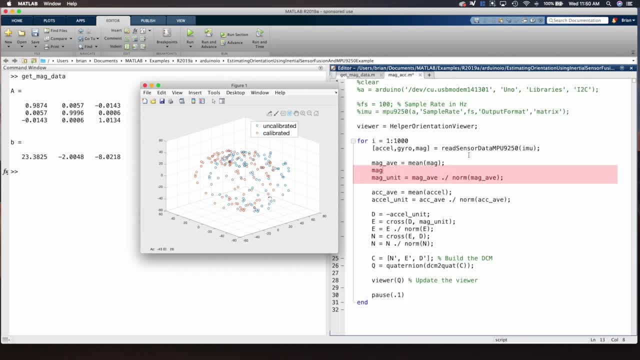 that I showed you previously, and a B matrix that will remove hard iron bias. I can add a calibration step to the fusion algorithm that I showed you previously, and this will produce a more accurate result than what I had before. and this will produce a more accurate result than what I had before. 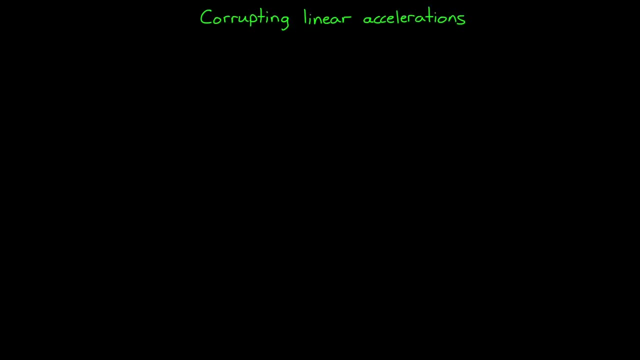 Alright, now let's go back to solving the other problem of the corrupting linear accelerations, and one way to address this is by predicting linear acceleration. and One way to address this is by predicting linear acceleration and removing it from the measurement prior to using it. And this might sound difficult to do, but it is possible if the acceleration error. 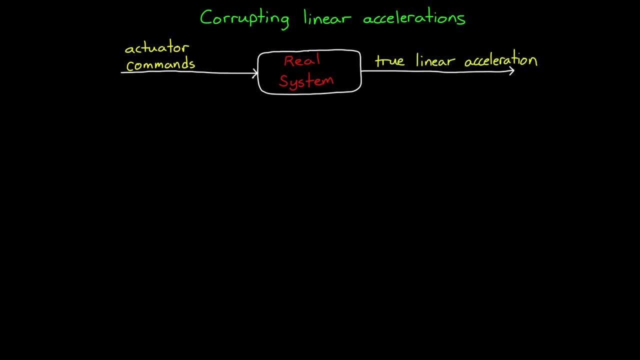 accessible� einfach. the acceleration is the result of the system actuators, you know, rather than an unpredictable external disturbance. What we can do is take the commands that are sent to the actuators and play it through a model of the system to estimate the expected linear acceleration. 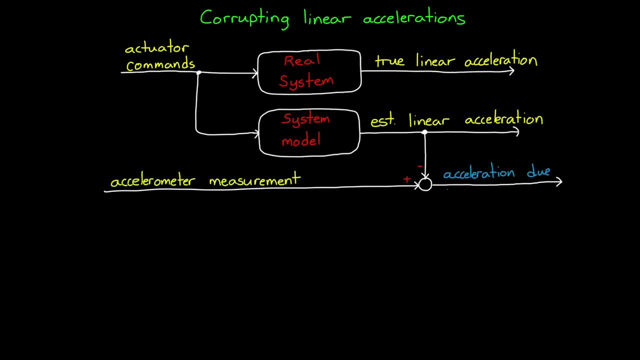 and then subtract that value from the measurement. This is something that is possible if, say, your system is a drone and you're flying it around by commanding the four propellers. Now, if we can't predict the linear acceleration or the external disturbances are too high, 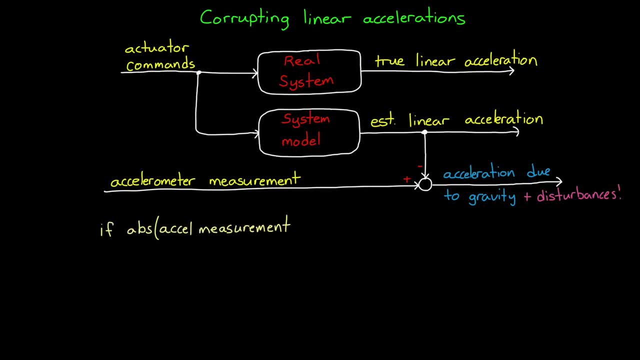 another option is to ignore accelerometer readings that are outside of some threshold from a 1G measurement. If the magnitude of the reading is not close to the magnitude of gravity, then clearly the sensor is picking up on other movement and it can't be trusted. 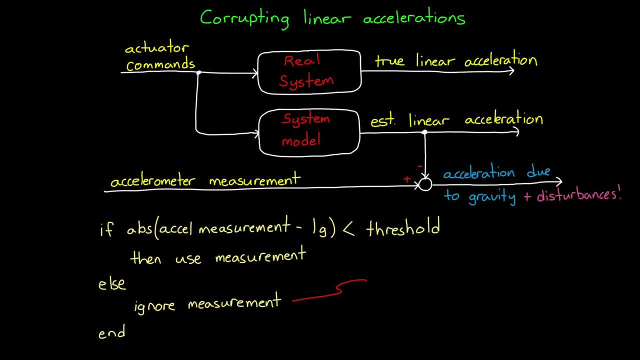 This keeps corrupted measurements from getting into our fusion algorithm, but it's not a great solution because we stop estimating orientation during these times and we lose track of the state of the system Again. it's not really a problem if we're trying to estimate orientation for a 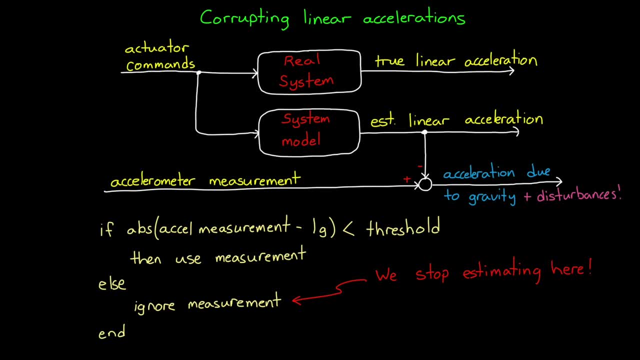 object. This algorithm would work perfectly fine. However, often we want to know the orientation of something that is rotating and accelerating, so we need something else here to help us out. What we can do is add a gyro into the mix to measure the angular rate of the system. 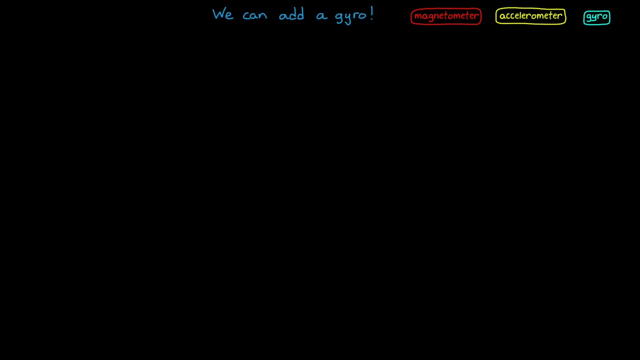 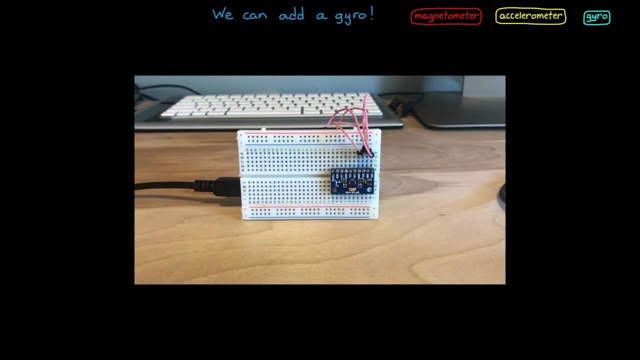 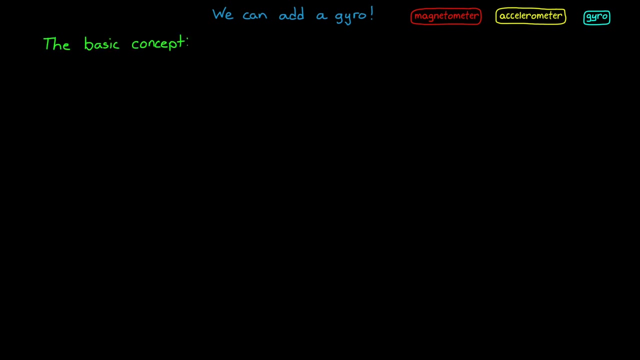 In fact, the combination of magnetometer, accelerometer and gyro are so popular that they're often packaged together as an inertial measurement unit, like I have with my MPU9250.. So the question is: how does the gyro help? To start, I think it's useful to think about how we can estimate orientation for a rotating object. 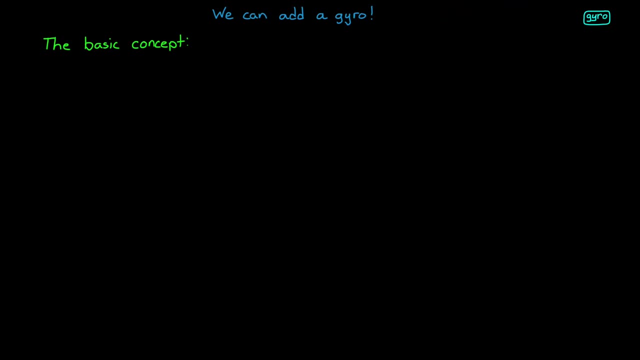 with just the gyro on its own, No accelerometer and no magnetometer For this. we can multiply the angular rate measurement by the sample time to get the change in angle during that time, And then if we knew the orientation of the phone at the previous sample time. 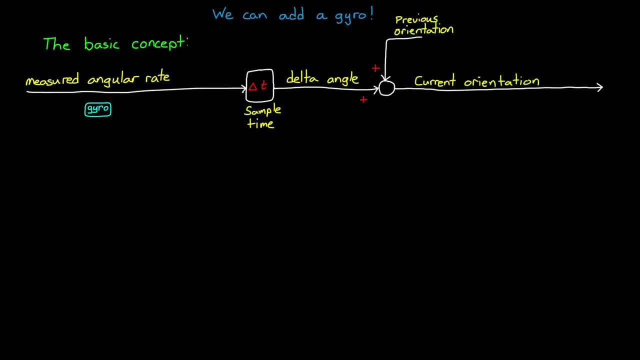 we could just add this delta angle to it and have an updated estimate of the current orientation, And if the object isn't rotating, then the delta angle would be zero And the orientation wouldn't change. so it all works out, And by repeating this process for the next sample time and the one after that. 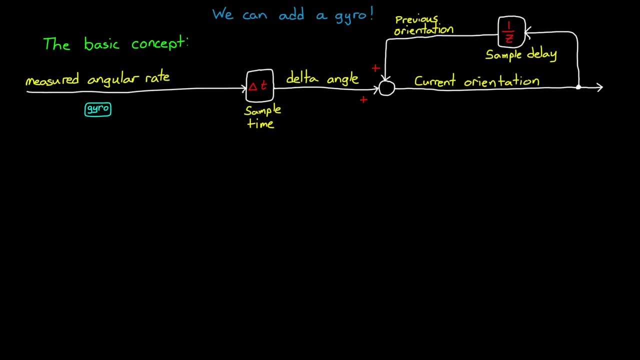 we're going to know the orientation of the phone over time. This process is called dead reckoning and essentially it's just integrating the gyro measurement. Now there are downsides to dead reckoning. One: you still need to know the initial orientation before you begin, so we need to figure that out. 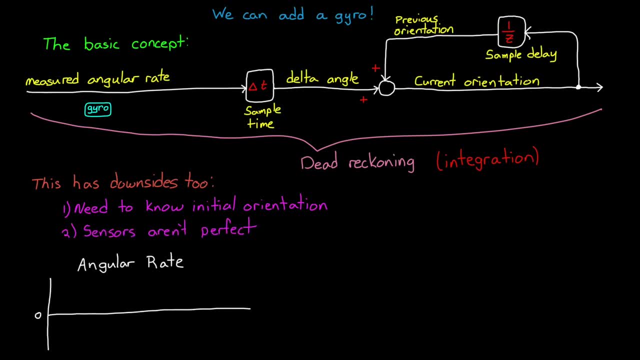 And two sensors aren't perfect. They have bias. Another, high frequency noises that will corrupt our estimation. Now, integration acts like a low pass filter, so that high frequency noise is smoothed out a little bit, which is good, but the result drifts away from the true position due to random walk as well as 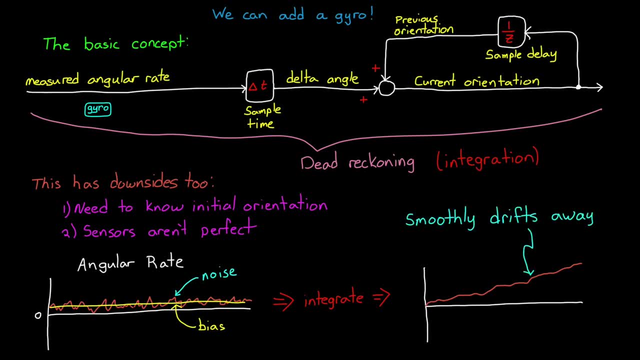 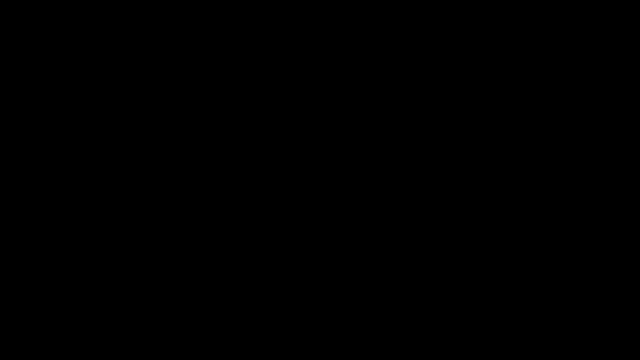 integrating any bias in the measurements. So over time the orientation will smoothly drift away from the truth. So at this point we have two different ways to estimate orientation, one using the accelerometer and the other using just the gyro, and each way have their own respective benefits and problems. 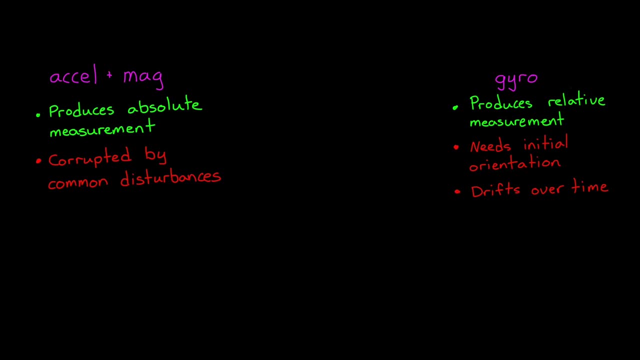 And this is where sensor fusion comes in once again. We can use it to combine these two estimates in a way that emphasizes each of their strengths and minimizes their weaknesses. Now there's a number of sensor fusion algorithms that we can use like a complementary filter or a Kalman filter, or the more specialized but common Madgwick or Mahoney filters. 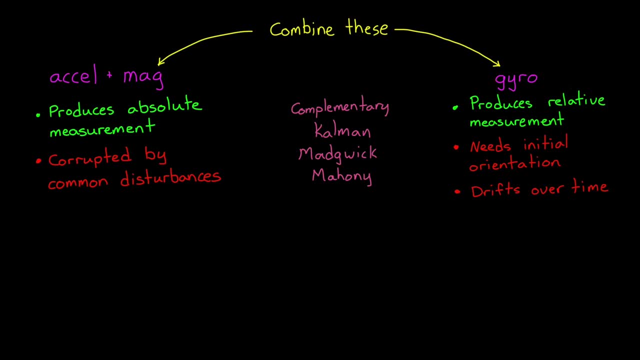 But at their core, every one of them does essentially the same thing. They initialize the attitude either by setting it manually or using the initial results of the Mag and accelerometer, And then, over time, they use the direction of the Mag field and gravity to slowly correct for the drift in the gyro. 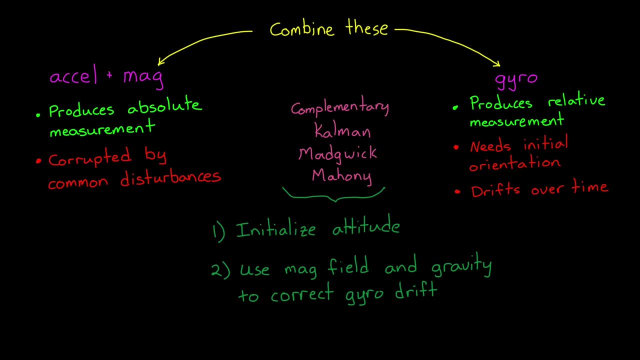 Now I go into a lot more detail on this in my video on the complementary filter, and MathWorks has a series on the mechanics of the Kalman filter. Both are linked below, But just in case you don't go, Go And watch them right away. 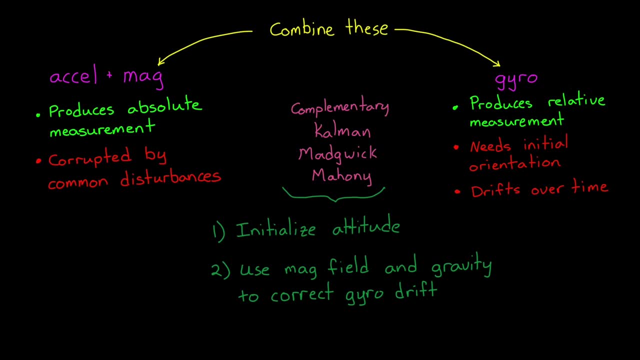 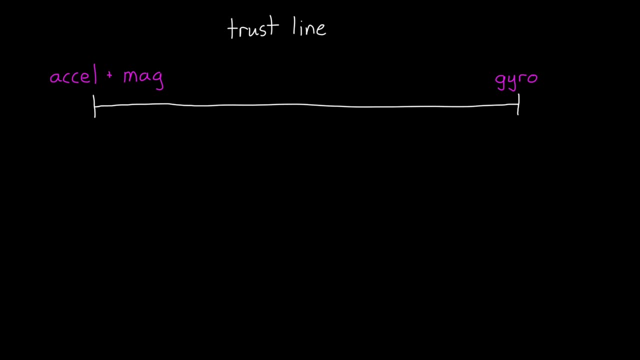 Let me go over a really high level concept of how this blending works. Let's put our two solutions at opposite ends of a scale that represents our trust in each one and we can place a slider that specifies which solution we trust more. If the slider is all the way to the left, then we trust our Mag and Excel solution 100 percent and we just use that value for our orientation all the way to the right and we use the dead reckoning solution 100 percent. 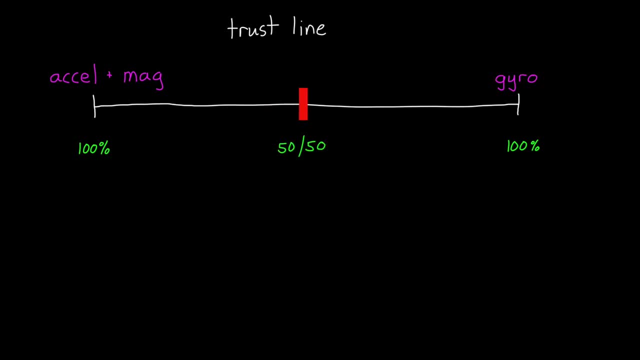 When the slider is in between. this is saying that we trust both solutions some amount and therefore want to take a portion of one and add it to the complementary portion of the other By putting the slider almost entirely to the dead reckoning solution. we're mostly trusting the smoothness and quick updates of the integrated gyro measurements, which gives us good estimates during rotations and linear accelerations. 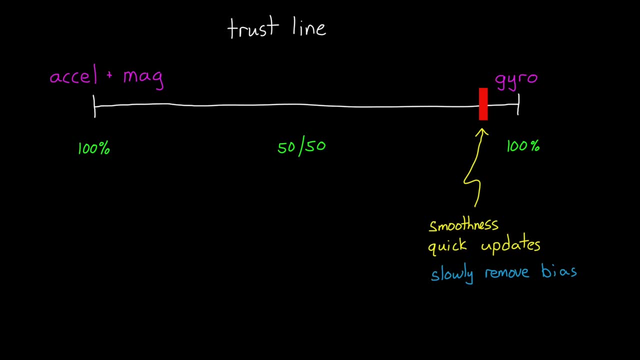 But we are ever so gently correcting that solution back towards the absolute measurement of the Mag and Excel To remove the bias before it has a chance to grow too large. So these two approaches complement each other. Now for the complementary filter. you, as the designer, figure out manually where to place this slider, how much you trust one measurement over the other. 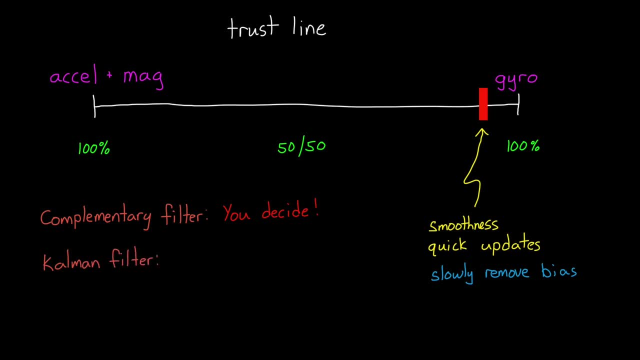 But with a Kalman filter the optimal gain or the optimal position of the slider is calculated for you after you specify things like how much noise there is in the measurements and how good you think your system model is. So the bottom line is that